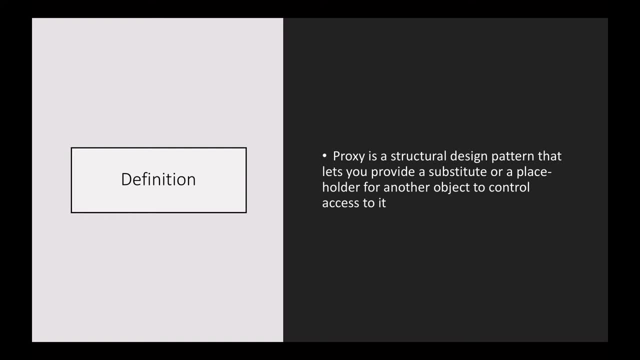 object provides. What this placeholder object does is. it can do the validation for you whether actually the inputs you are giving or you are about to give to the objects are valid or not, and based on that you could actually reject or continue the behavior. The benefit with this? 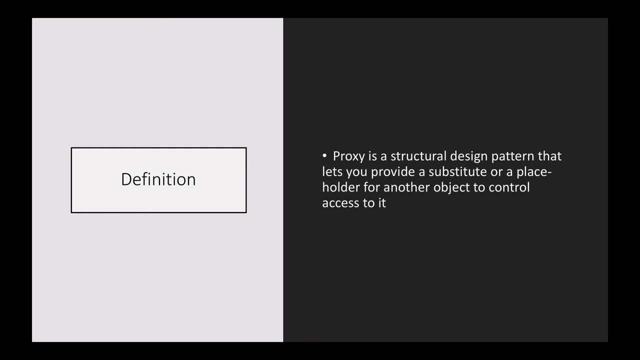 approach is, whenever you are using a proxy, this- all this pre-instantiation and prerequisite code is not actually scattered in your code base. It sits at one place. and it is not scattered in your code base. It sits at one place inside the proxy object. So whenever you want to talk to the actual object, 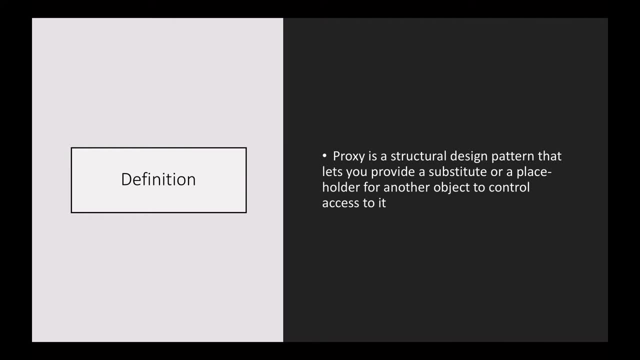 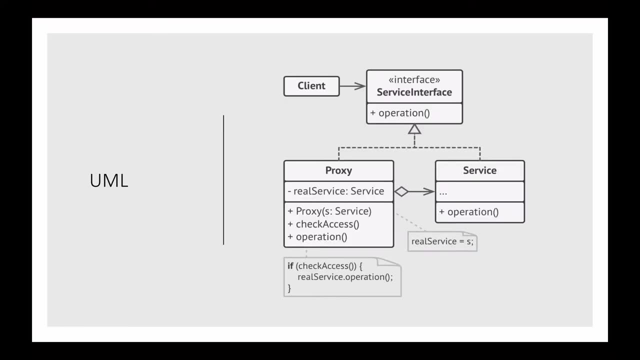 which is a very high consumption and resource taking object, you wrap it in a proxy and then give it to the client. Let's take a look at the UML diagram. So in the UML diagram the client is actually needing a service interface which has some operation. let's say Now, let's assume that 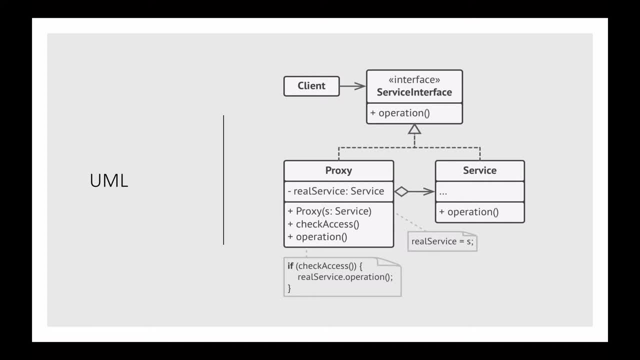 this operation is very, very, very expensive to perform and even invalid inputs. this operation can take a heavy number of resources and actually fail, which is not expected. So what we do is for this service, we abstract this operation in an interface called service interface and then we derive two implementations for this interface. One is the 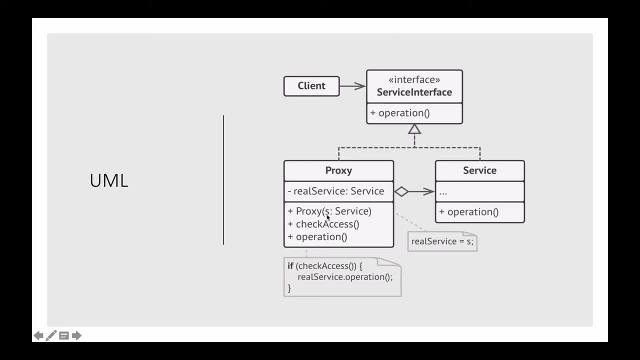 service itself and the other one is the proxy service. So this proxy service will actually have a reference to the actual service it is trying to target And in the constructor you can actually instantiate this proxy with a service of any type you want. And this proxy, since it is implementing the same interface as the service itself, it will also have those. 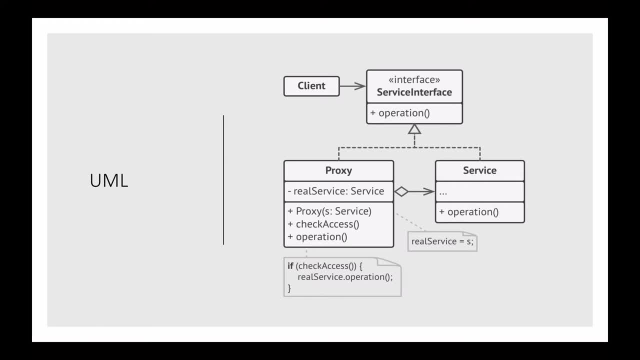 operations in the background and we can actually have some pre-processing logic before calling the actual service in the proxy. So this is what proxy pattern is trying to do: it is trying to pre-process your inputs before actually Calling the actual target service. Let's take a look at the coding example. The coding example. 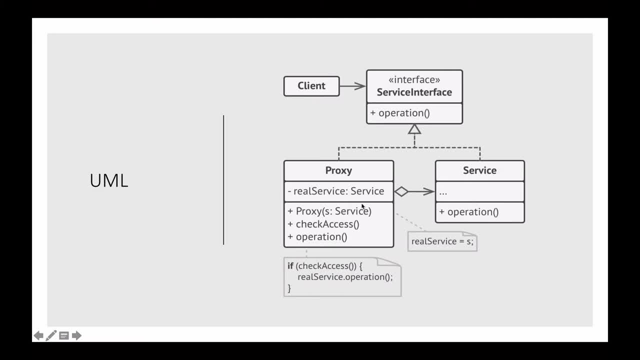 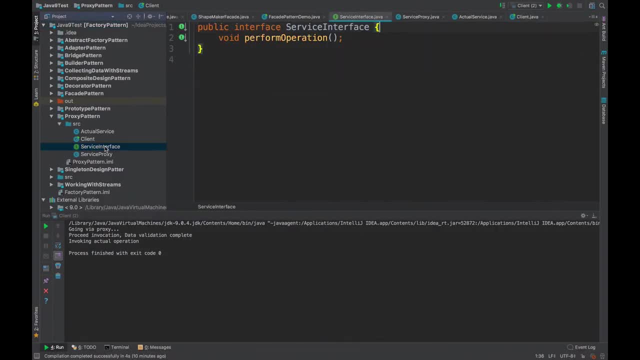 I have written is inspired from this UML diagram, So you will find a very direct similarity between the UML diagram and the coding example. Here we have the coding example, So let's go to our service interface. This is a very small interface which has only one operation called the perform operation. So 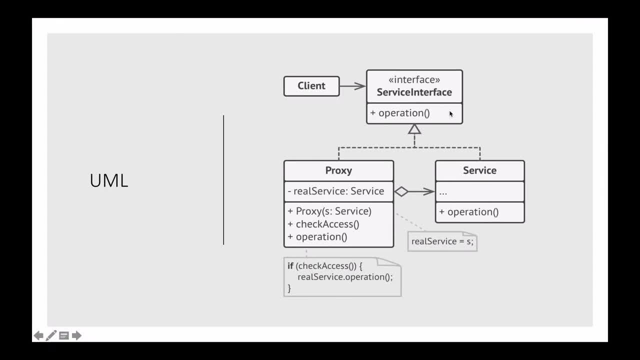 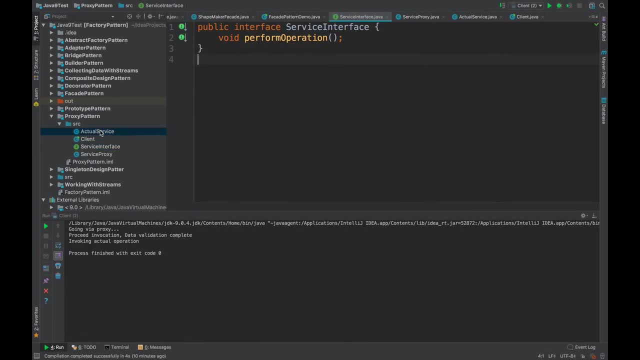 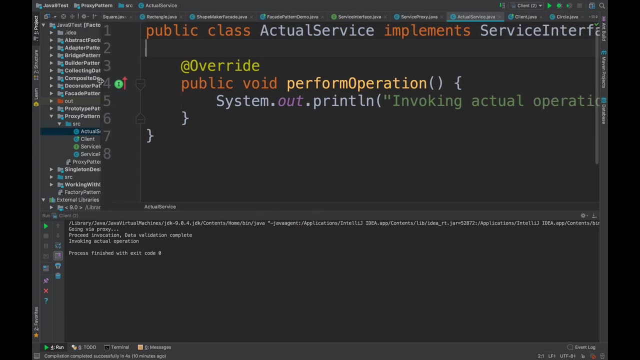 and There are two implementations for this Service interface. one is the service itself and the other one is proxy. So let's go to the service itself and I have named it actual service. so let me remove the borders so you will be able to see what's happening here and 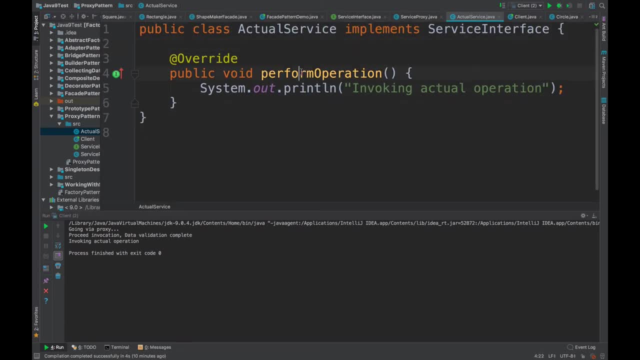 in the actual service. what I'm trying to do is actually I am giving a Behavior to this perform operation. I'm giving it a method body. in this body, I'm trying to actually invoke the actual operation. and Let's assume that this operation is quite expensive and we don't want to actually 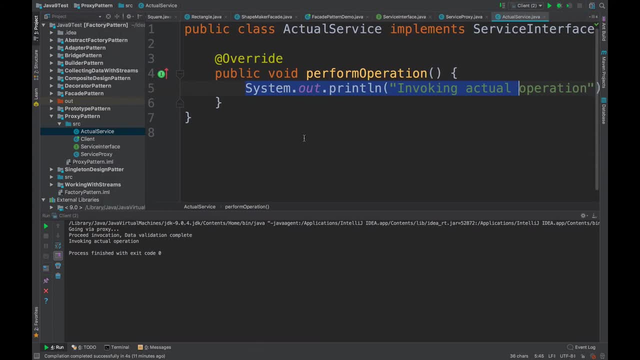 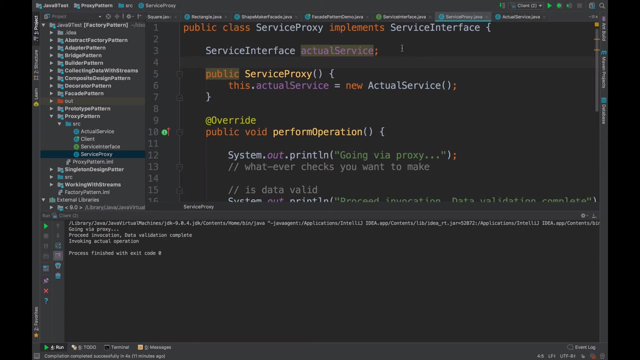 Just directly go and invoke this operation. We want some prerequisites to be checked. So for the prerequisites class, I have created this service proxy Which actually implements the same service interface and has a reference to the actual service. As you see, in the UML diagram we have a private reference to the actual service and in the constructor 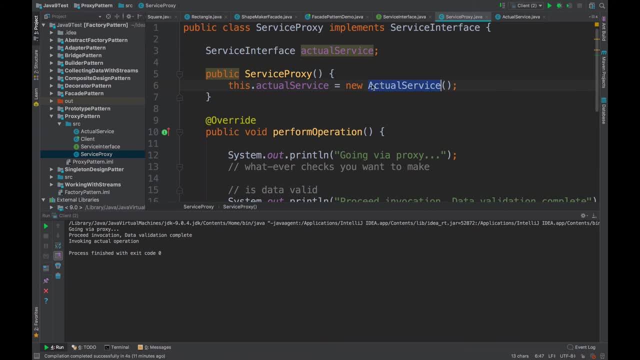 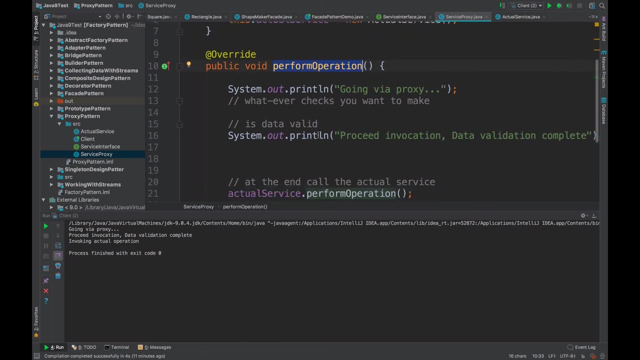 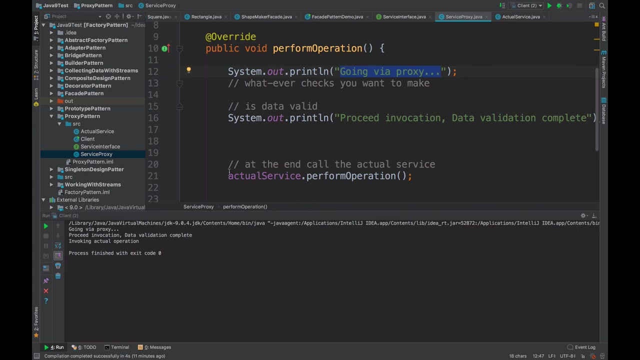 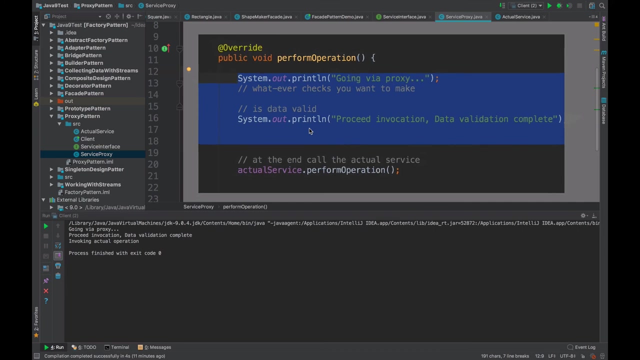 We are initializing the service. Similarly, in the constructor We are actually initializing the service. Now, in the perform operation method of this proxy object, we are logging some Texts which is going through proxy and before actually invoking the actual perform operation, You can do all the pre-processing logic here. So for demo purposes, for the pre-processing logic, 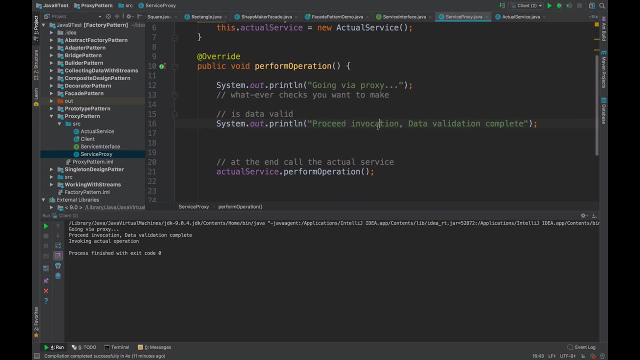 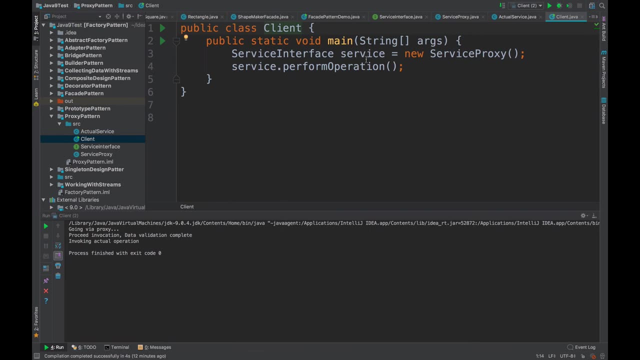 What I am doing here is just printing out some println statements, which is proceed, invocation Data validation complete. So whenever this client wants a proxy Service, we give it a proxy, and this proxy can be decided through a factory pattern And we have discussed it in the creational design pattern series. 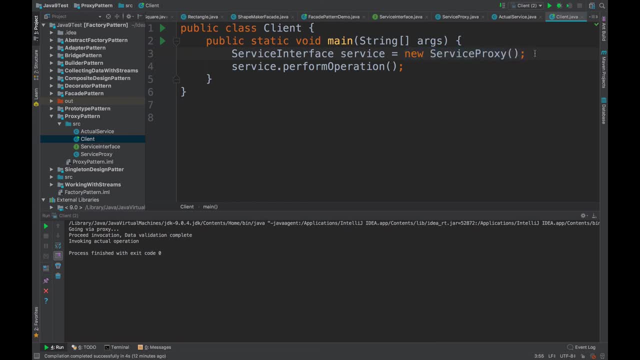 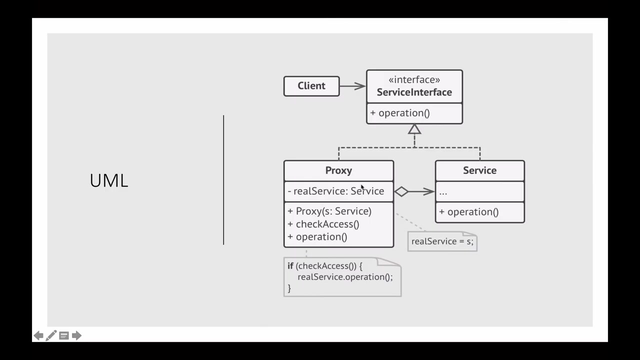 So if you have not watched it, you could just you can just go and check it out. so service interface will have a reference to a proxy and the proxy will perform the all the prerequisites which are needed to actually invoke the operation in the actual service. This is the problem It is trying to solve and we have seen how it is trying to solve the problem. 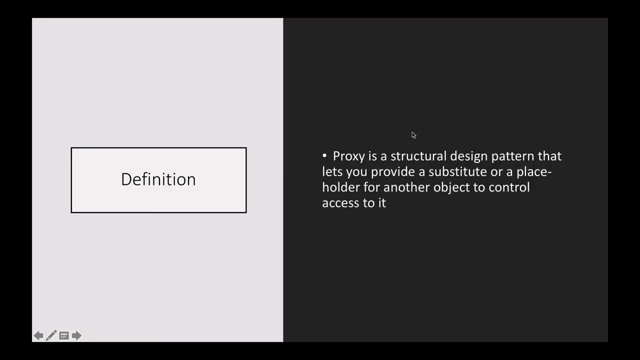 So this is the intent of the proxy design pattern. Let's take a look at the definition again. Proxy is a structural design pattern that lets you provide a substitute or a placeholder for another object to control access to it. Now you know. why do you need a substitute, What is a substitute and how to use it.